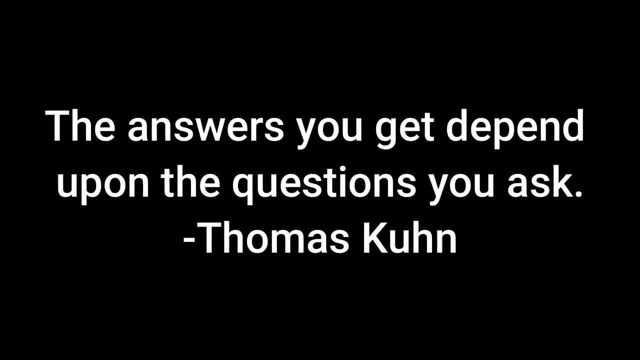 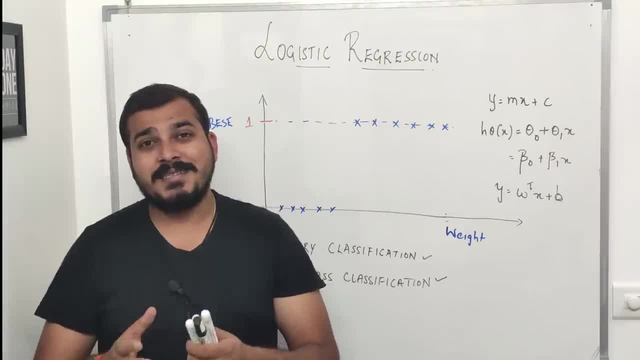 Hello all my name is Krishnak and welcome to my YouTube channel. Guys, this is the 35th tutorial in complete machine learning playlist and I have promised you guys I will be completing all the machine learning algorithms. There are around some 50-20 machine learning algorithms. 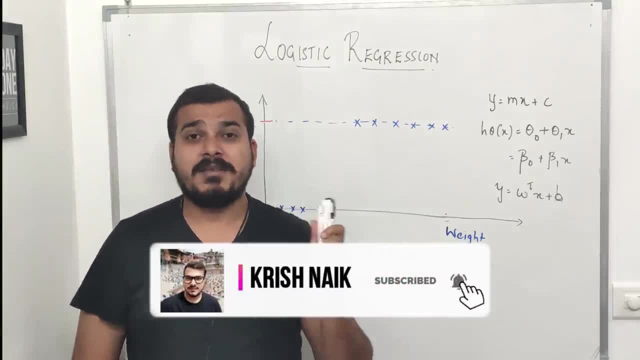 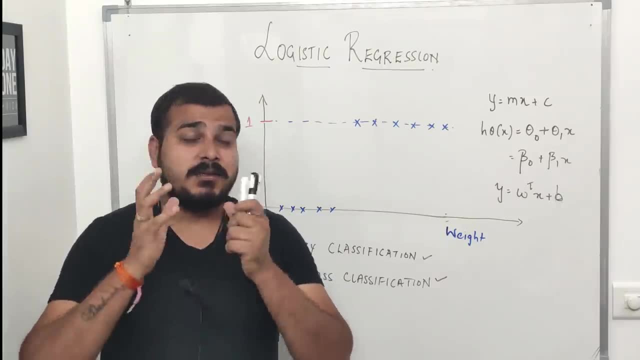 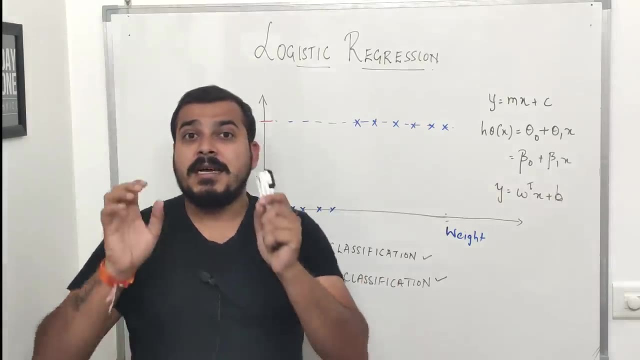 which I will be completing and uploading in my specific playlist that is called as complete machine learning playlist. Similarly, I have plans to upload the remaining videos in deep learning playlist also- and this was one of the most requested- and you wanted the in-depth intuition Why I am actually uploading these particular videos, guys. is that to explain? 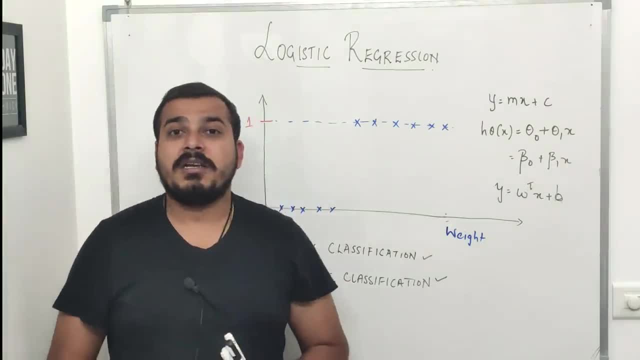 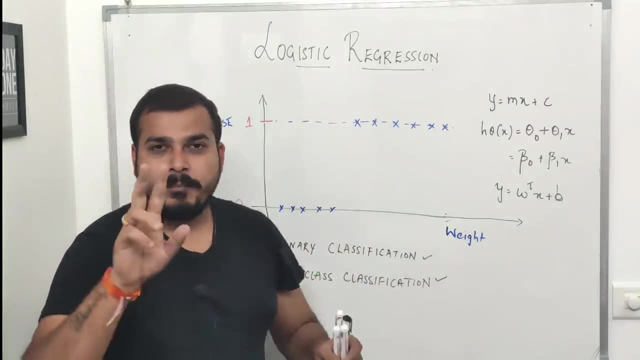 you the complete maths. what is the maths behind the machine learning algorithms? and some of the machine learning algorithms may go till some different parts. This is the part 1.. Suppose in logistic regression I am planning to complete it in part 2.. So part. 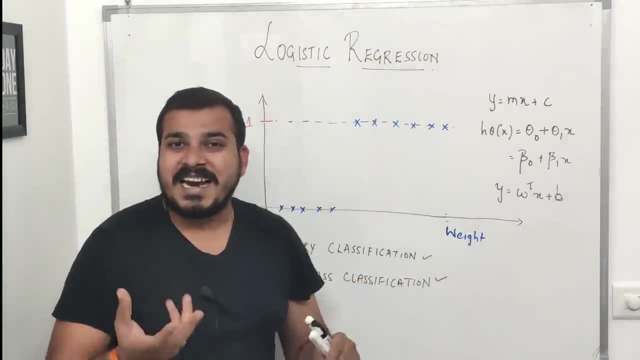 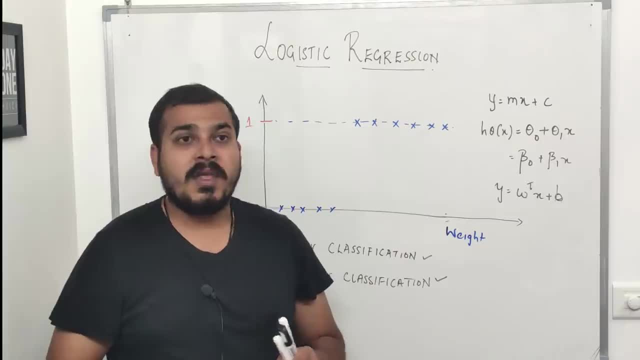 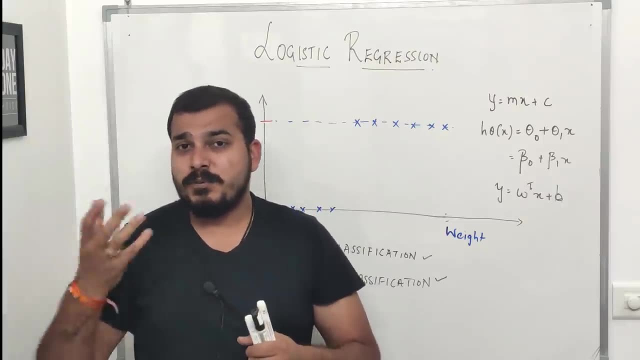 And in the part 2 we will understand the maths behind it. Here also we will be understanding some of the maths. Now, this intuition is pretty much important because, as you all know, that implementation with the help of Python, by using libraries like sklearn, is pretty much. 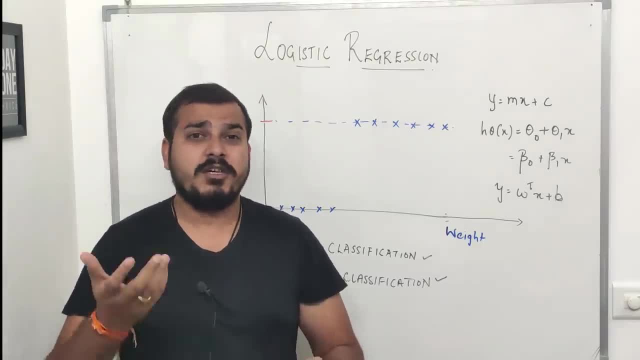 simple, and I have also shown you in many videos how you can actually do hyperparameter optimization and many more things. So it is very, very important to understand the maths behind that, because that will actually help you in doing the hyperparameter optimization and in the interview they need. 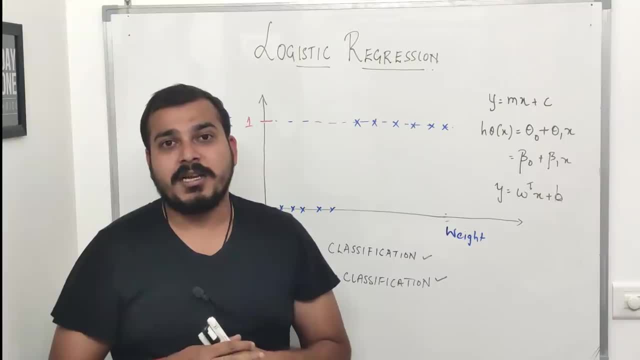 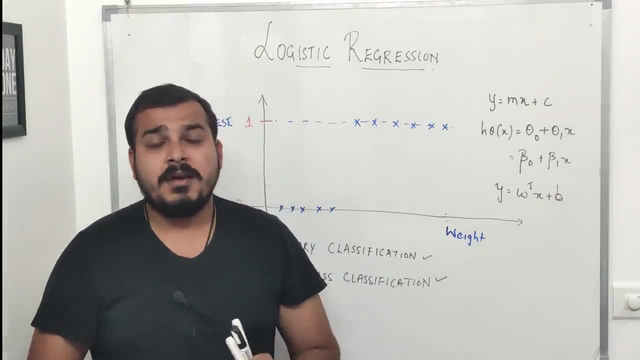 to basically ask you the maths behind this particular machine learning algorithm. So in this specific video we will try to understand about logistic regression. This will be divided into two parts. This is part 1. So make sure that you understand this particular video. 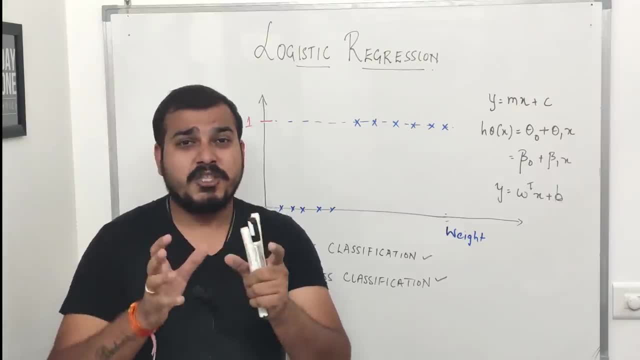 Now, guys, if you are looking for career transition advice towards data science, please make sure that you watch this particular video till the end, because I am going to share you some of the important things at the end of this particular video. So let us go ahead and try. 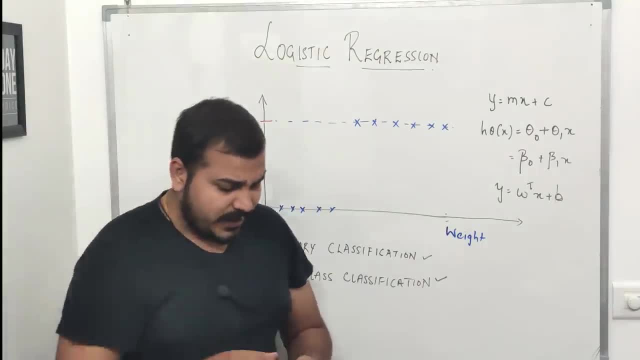 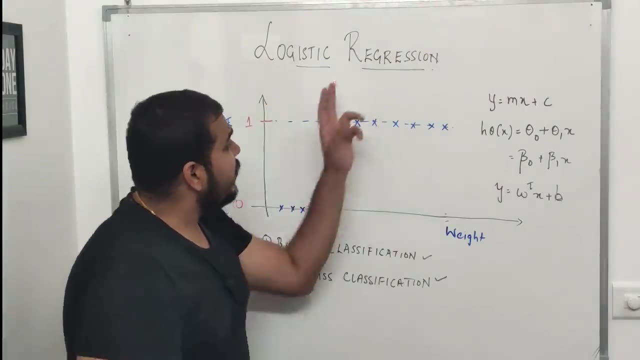 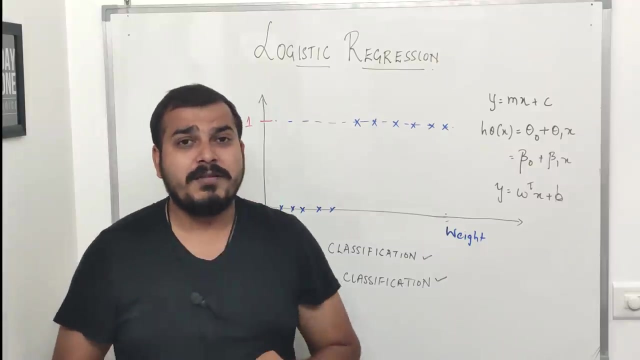 to understand. how does logistic regression actually work? Now, understand one thing, guys: First of all, why this algorithm is actually used. First of all, why this algorithm is actually used. This is a machine learning algorithm, So in logistic regression it is basically used for binary classification. Now I hope in my tutorial 31st I had actually uploaded videos. 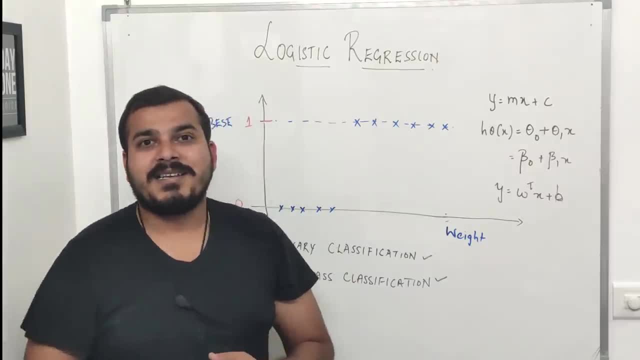 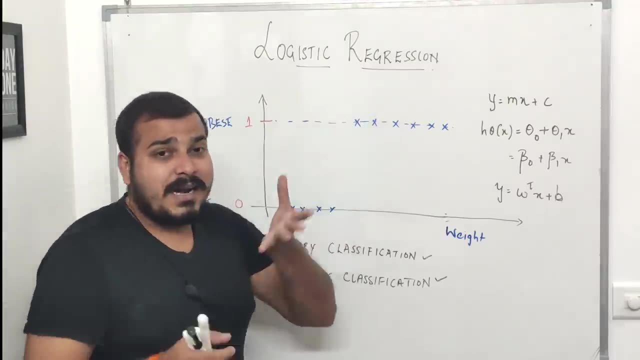 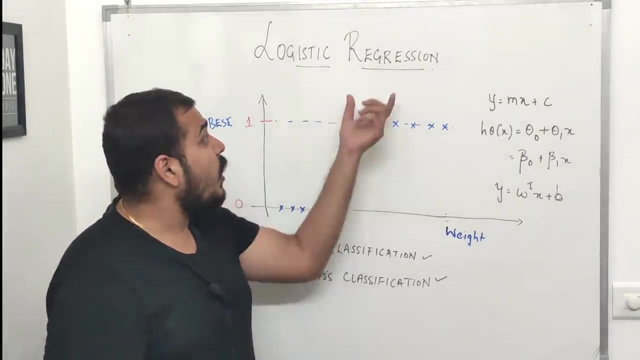 regarding linear regression and we understood the various metrics like R squared, R squared, errors, everything we tried to understand in that. But in binary classification now that was a regression kind of problem statement. Logistic regression is basically a binary classification problem statement. But why it is called as a regression? Because it is. 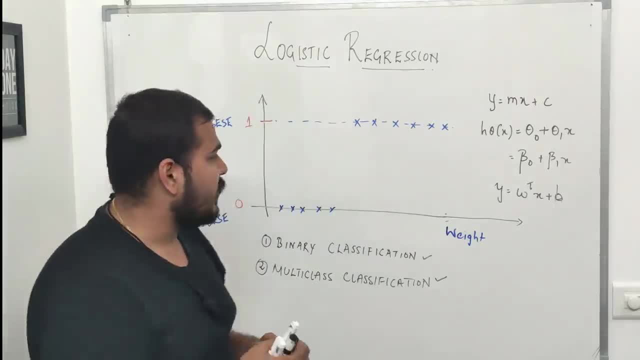 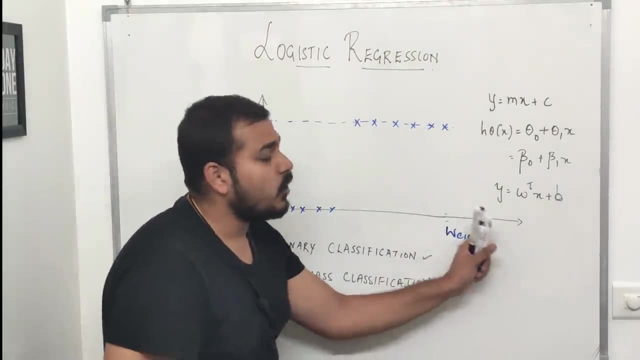 a binary classification problem statement. It is a binary classification problem statement. Okay, Now see, very important thing over here is that. let me take a very, very simple use case. Now, in my y, in my x axis, I have a parameter called as weight. So this is my x value. Okay, 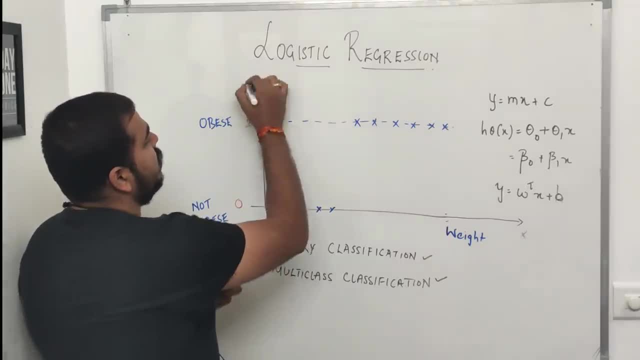 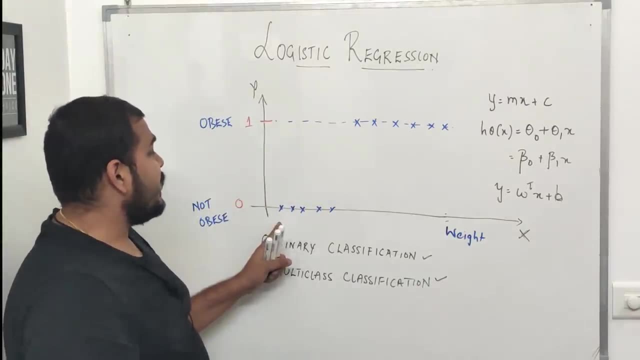 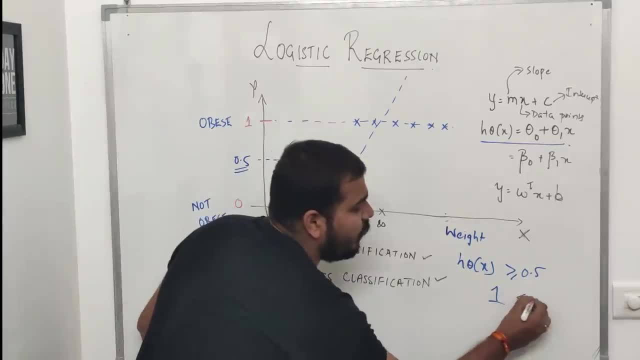 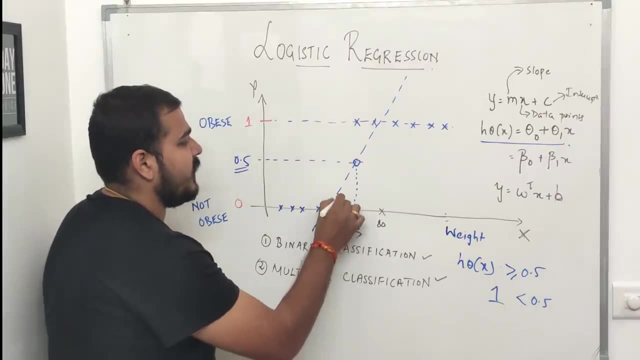 way is actually obese, right? if it is less than 0.05, then it will become not obese. so that basically means, suppose, if I'm considering this way, 60 kg and if I just try to populate this, right? oh sorry over here, so this will be my probability. 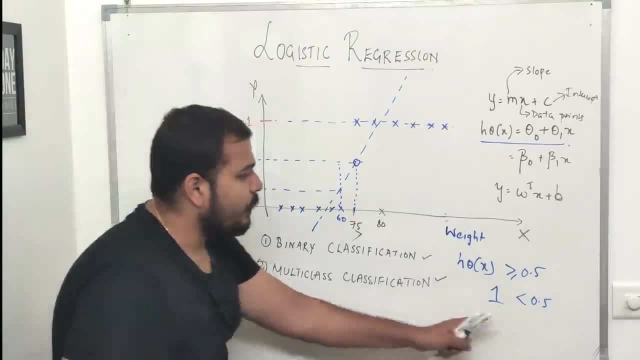 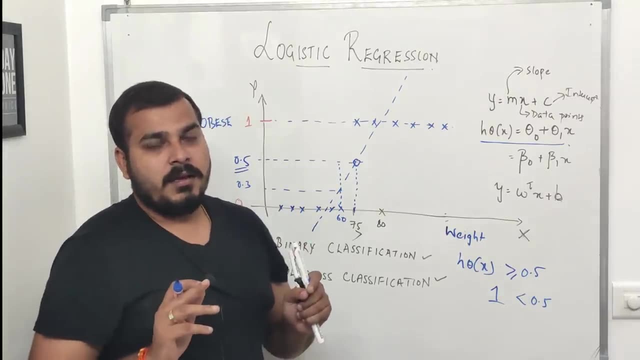 value that I'll get, suppose this is 0.3, right, so it is less than 0.5. so I'm going to consider that 60 kg that person is going to become, not obese, right? pretty much simple now. with the help of this straight line, I am able to classify. 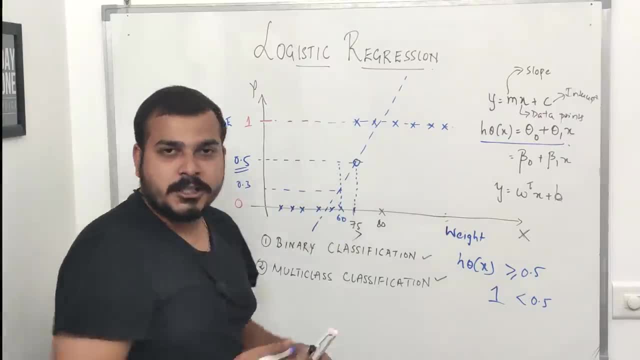 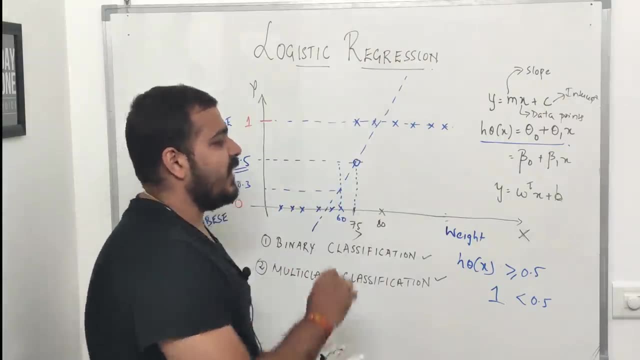 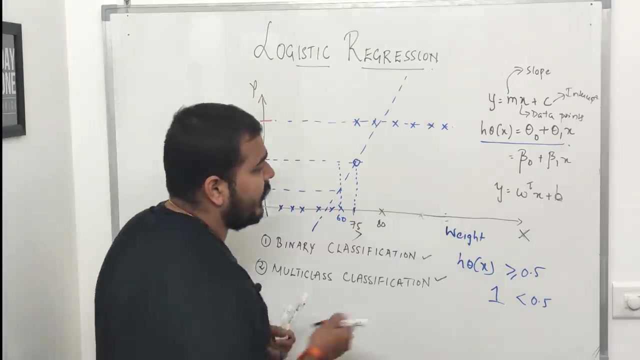 easily right. so what is the use of logistic regression? that is the next question that comes up right. it is pretty much important to understand. you can see over here by just creating a straight line. now suppose my new data point comes over here. okay, sorry for this. suppose my new data points comes. 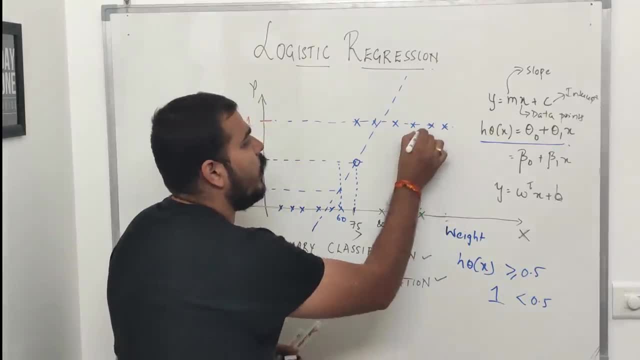 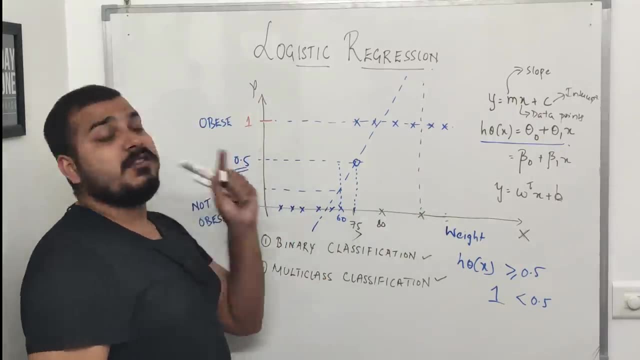 over here. now you need to find out. I'll just go and connect this particular point. now it is greater than 0.5. I can definitely say that this person is not obese. sorry, this person is obese. suppose if I want to find out a new value over here, I may. go over here, I may. 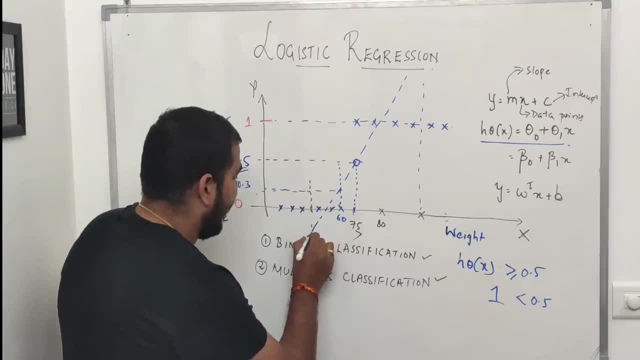 find out. this is my sorry, it will be negative value, okay, so somewhere over here it is less than 0.5, so I'm going to consider that the person is not obese, right? and this gets extended over here, right, guys? so I can find out this. 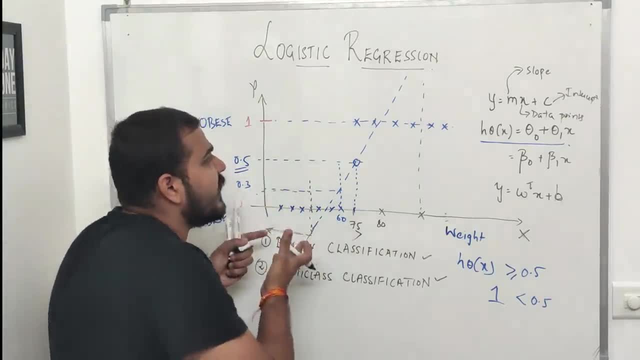 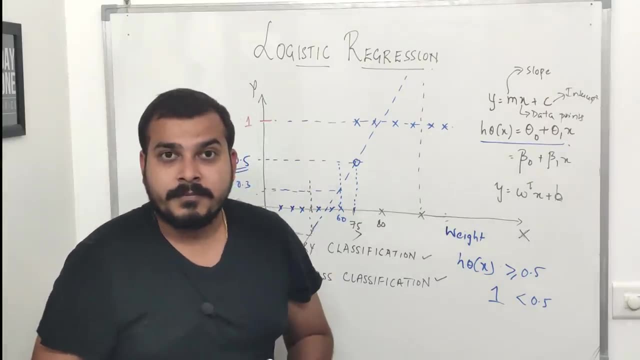 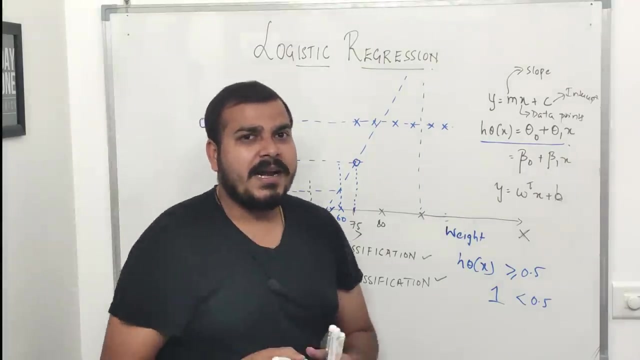 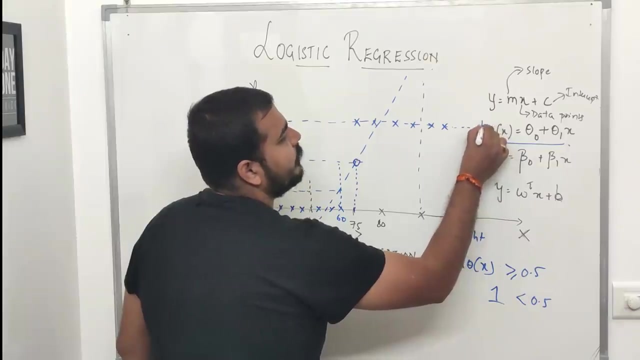 particular point, it will be negative. so just by considering a straight line I can solve the classification problem. so why exactly do we need the logistic regression now? understand one thing now. suppose I say that there is one more outlier added to it. suppose my outlier is somewhere here. just consider this: my outlier has come somewhere here. 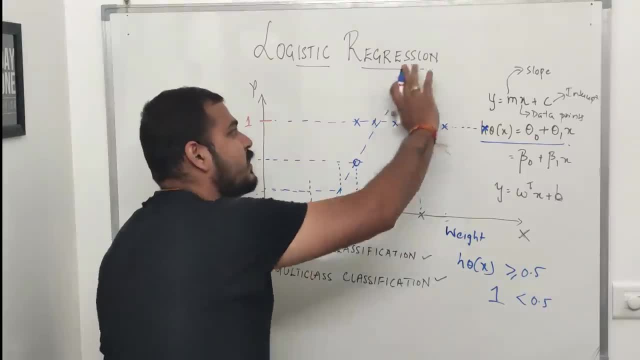 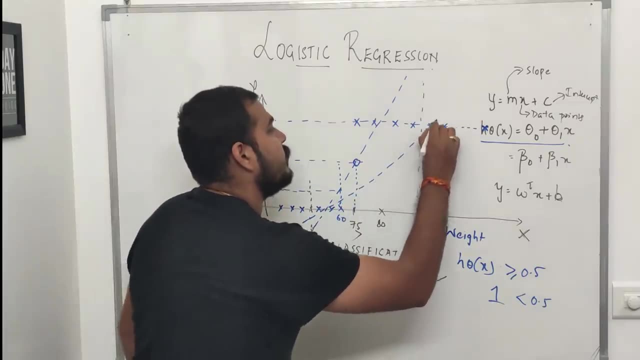 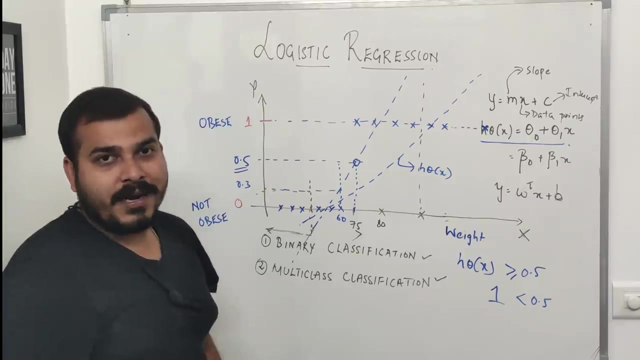 right now, if I try to create this best fit line once again, what will happen? this best fit line will now change. it will become something like this: right now, this is my new best fit line: S theta of X. right S theta of X. this is my new best fit line. but now understand this problem. statement, guys. we know that. 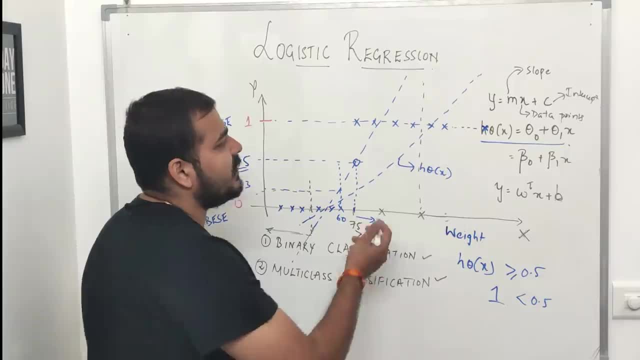 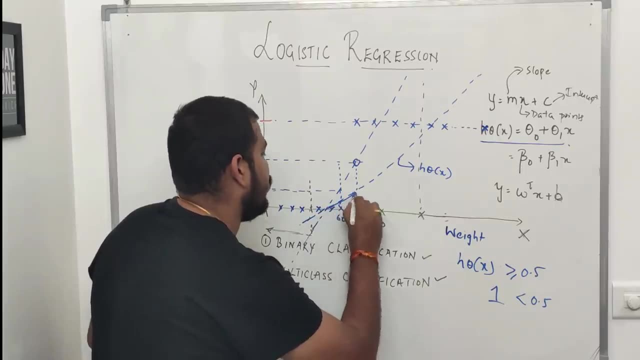 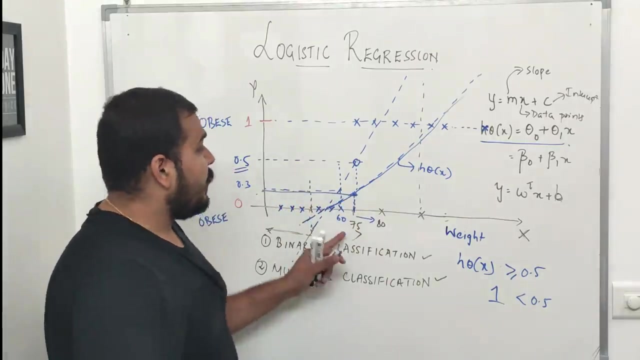 if the person is greater than 75 kg, we should classify this as obese category. but now if I go and see my 75% with respect to this best fit line that I have, it is coming somewhere over here. my 0.3 now that basically means that a person is not obese. 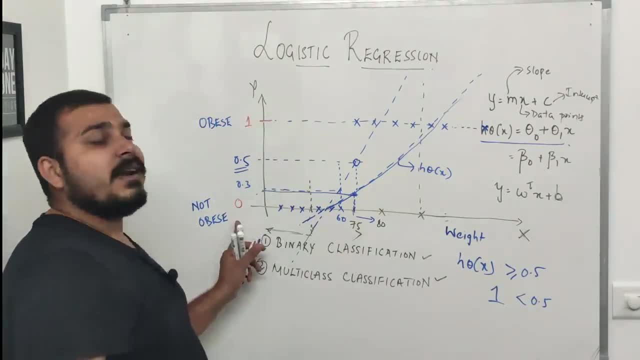 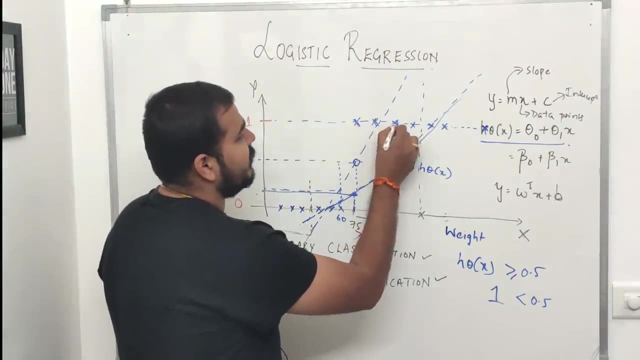 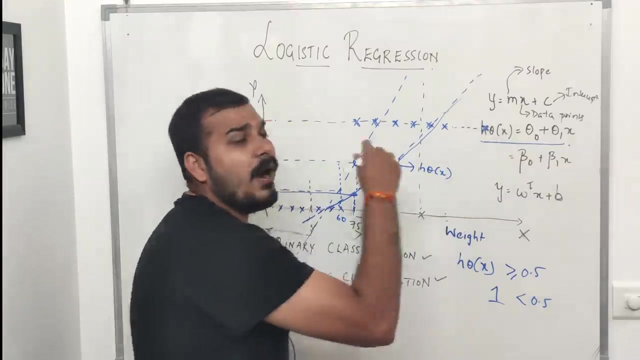 right now, if I go and see my 75 kg, right is clearly not obese. but this is, this was not what the result we actually wanted. right, because we clearly know that this particular point in my training data is basically having obese category. but first, by just the inclusion of one outlier, one point, the whole straight line. 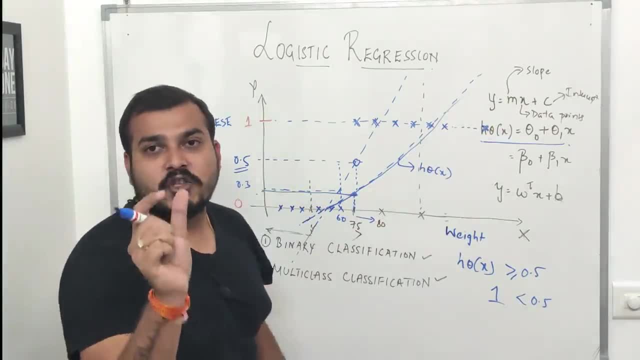 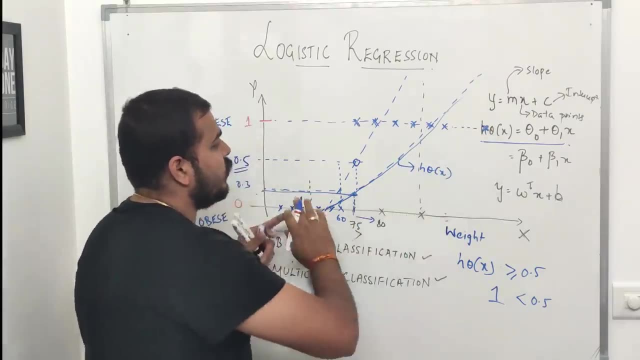 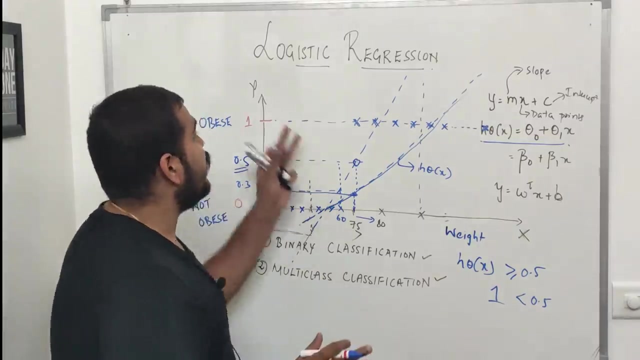 became deviated because this is the best fit line and this is actually computed based on the distance. right now, you have understood that because of the standard this, this whole best fit line has changed and because of that there is a high error rate now. because of this, we should not use linear regression for 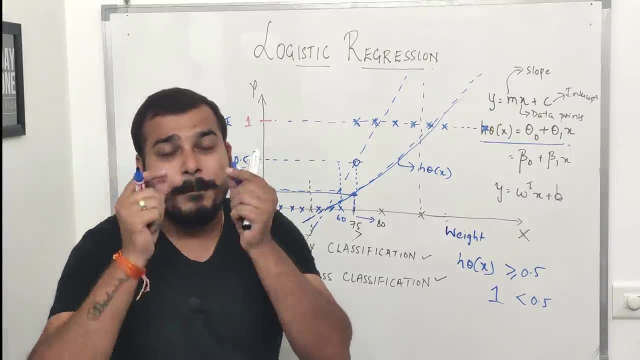 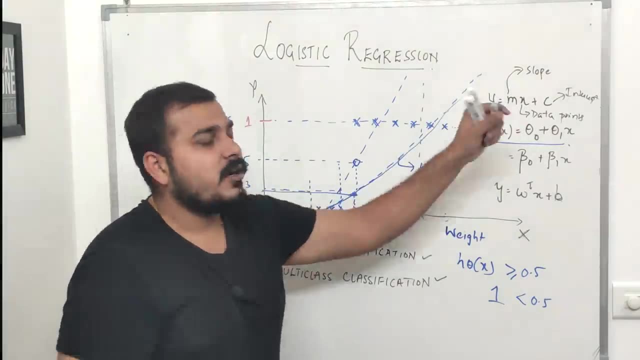 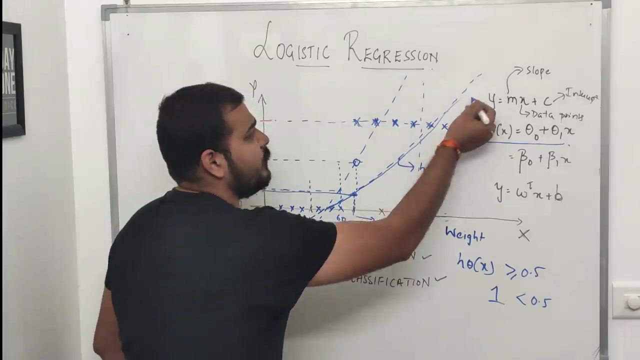 this kind of classification problem. now, this is the major, major problem with linear regression, because every time we have to create a best fit line based on the data points that we have and we know clearly that this particular points are obese. but with the help of this best fit line, what has happened now? suppose, if I 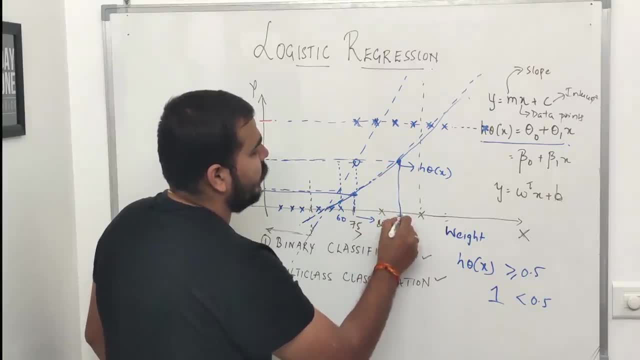 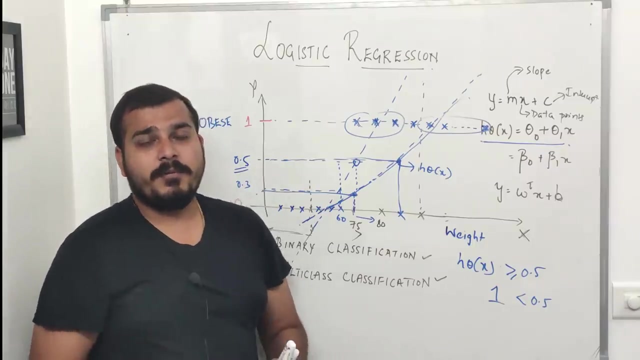 take this 0.5. it is pointed over here. I'll draw it over here. okay, so these all points will get incorrectly classified, right? so these are points will get correctly classified. that is fine, but these are points will get incorrectly classified, which is a very, very big problem over here, right? so because of 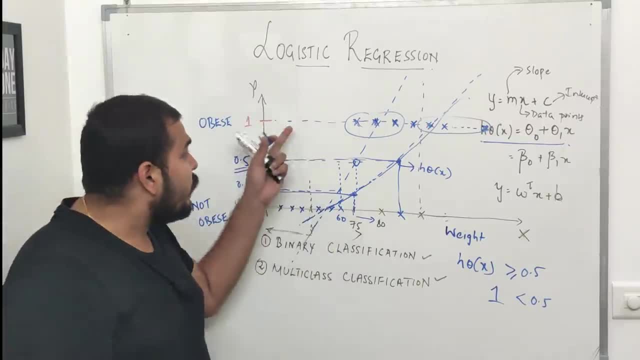 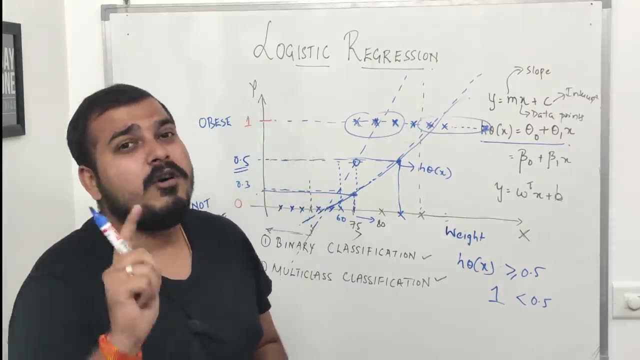 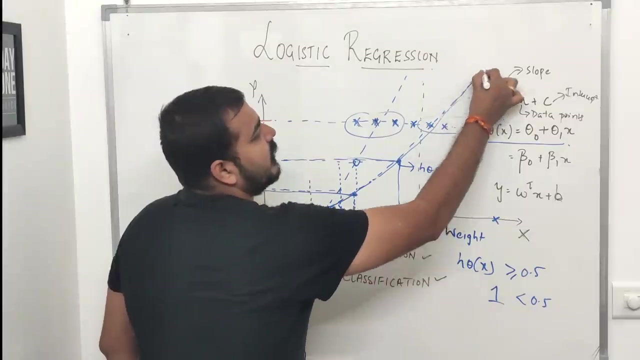 that we should never use linear regression for this particular binary classification. okay, then what should we do then? right, there is one more problem with linear regression. now understand over here, guys suppose my weight is somewhere here and this particular line is getting extended here. now, if I try to find out with 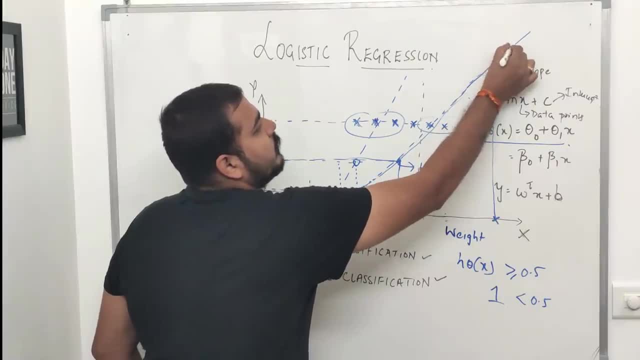 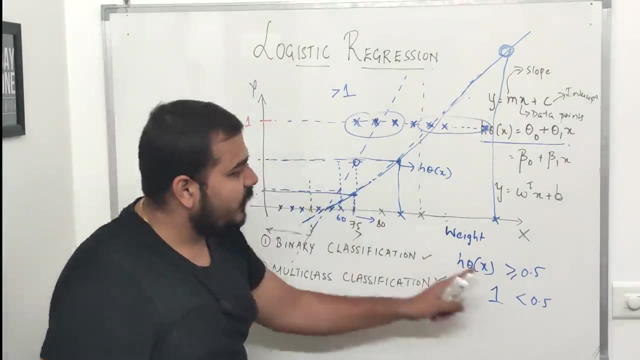 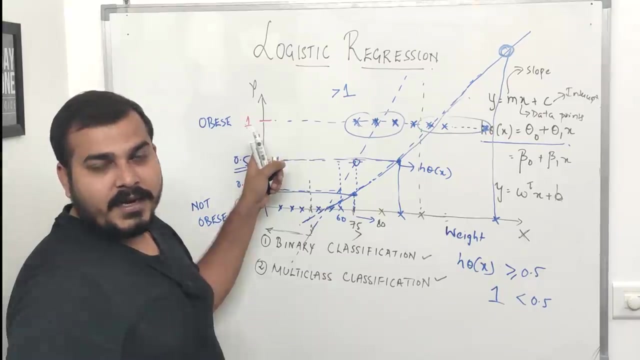 respect to this particular weight. what is my value right now? the answer is greater than 1. right, but we have told that if the value is greater than 0.5, okay, we are going to consider this. because the maximum value is 1, right, we are going to consider 1, but if it is, 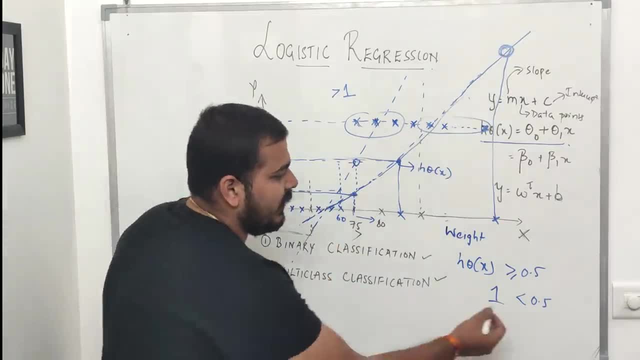 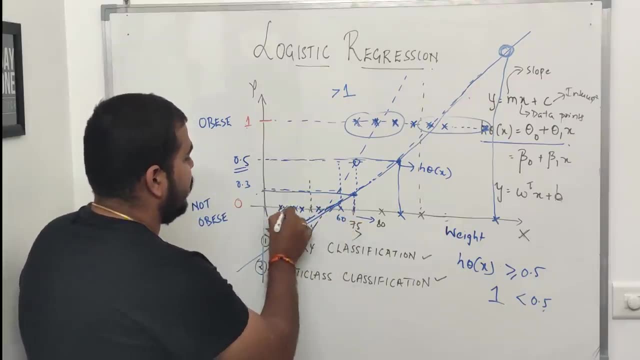 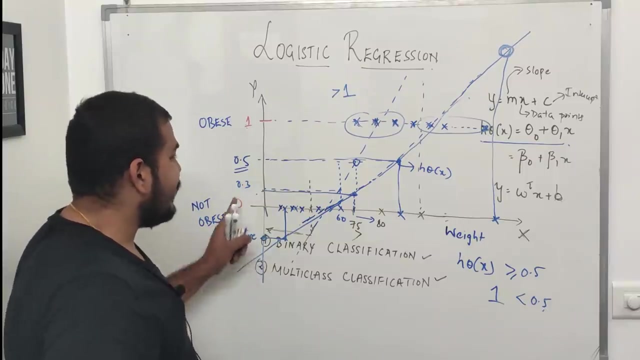 greater than 1, what do we consider now? similarly, if it is less than 0.5, suppose this is my point and, with respect to this, I am extending it downwards right now. suppose, if I consider this part, I tried to populate it. this is my negative value right now. when I have a negative value, weight is 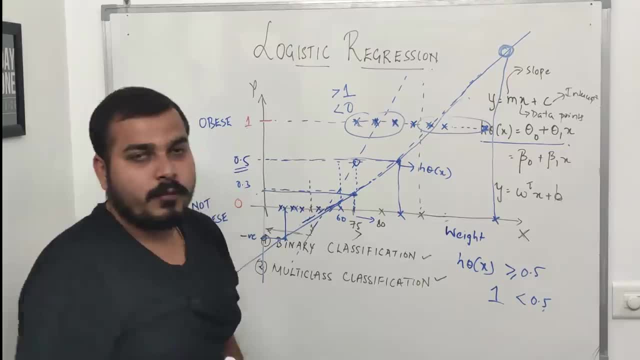 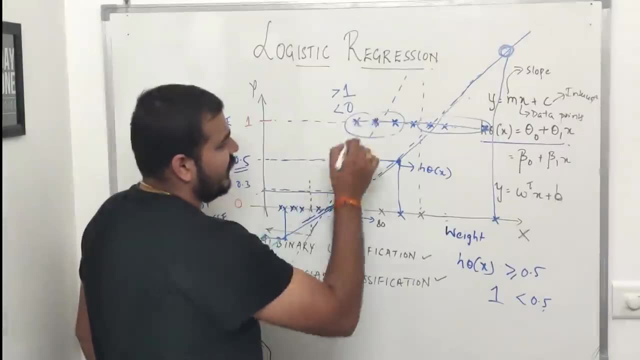 less than 0? what is greater than 1? one is less than 0. what do we consider for that? so instead, we should try to divide this, this line, like this: and this is basically done by a sigmoid function, which I will be explaining in my next class, because there will be lot of maths We have just understood. 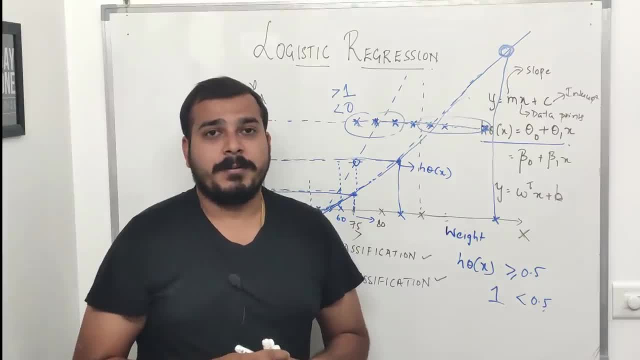 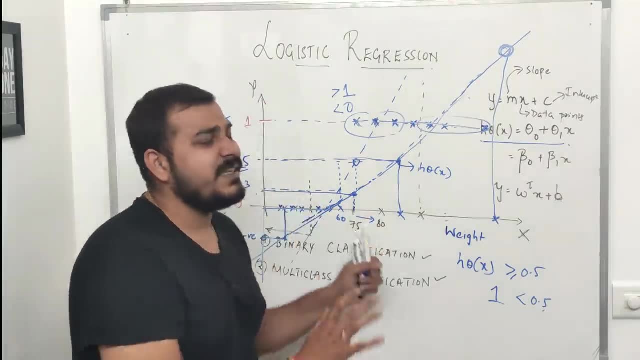 why linear regression will not work for this specific problem statement- And it will be interesting, guys, because I am going to include each and every bit of maths in a much more easy way so that you will be able to understand it. So two reasons why linear regression should. 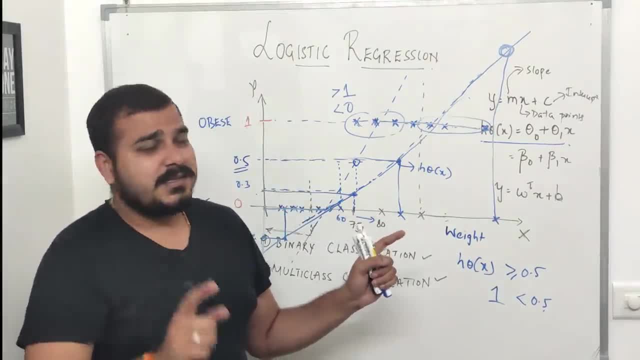 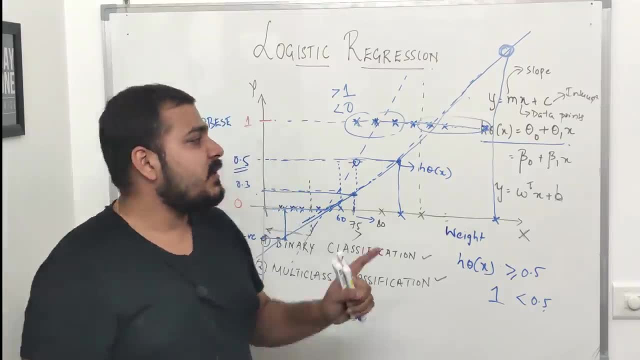 not be used for this binary classification guys. One is that whenever I have lot of points, lot of outliers, the best fit line will completely get deviated. The second thing is that whatever output I am getting, most of the time I am getting greater than 1, less than 0. So in 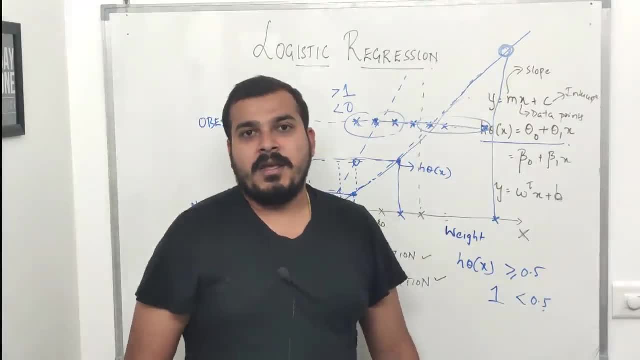 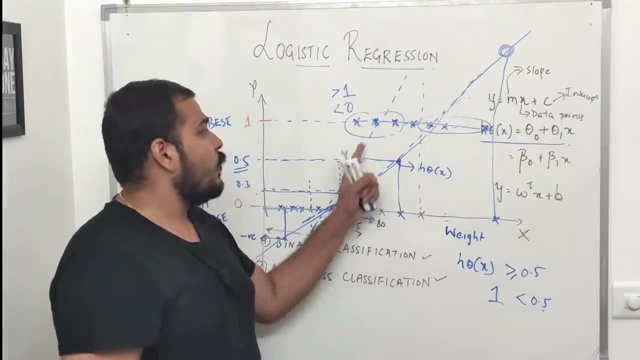 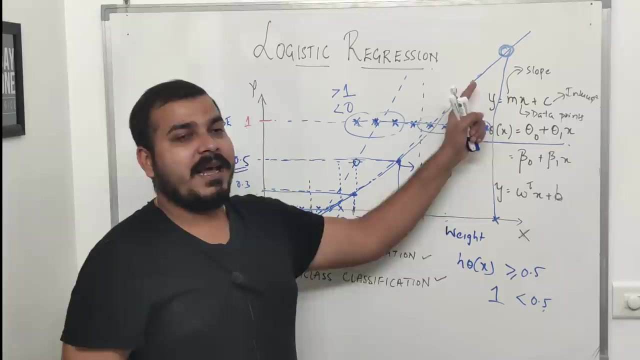 order to solve this particular problem, we have to use logistic regression, And logistic regression uses a very, very simple concept along with a function which is called a sigmoid function, which will squash this straight line, But before squashing, we need to understand how this best fit line. So, basically, if I 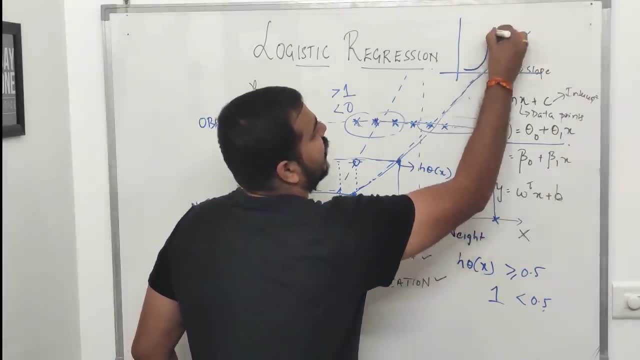 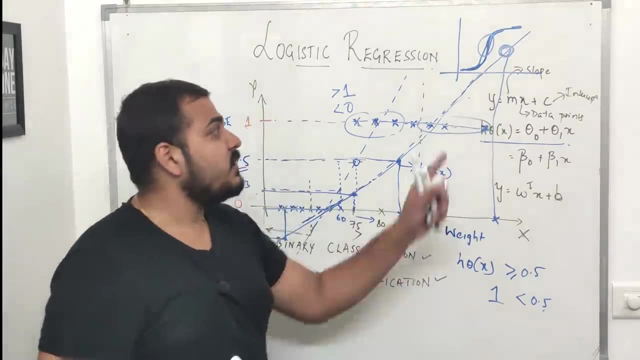 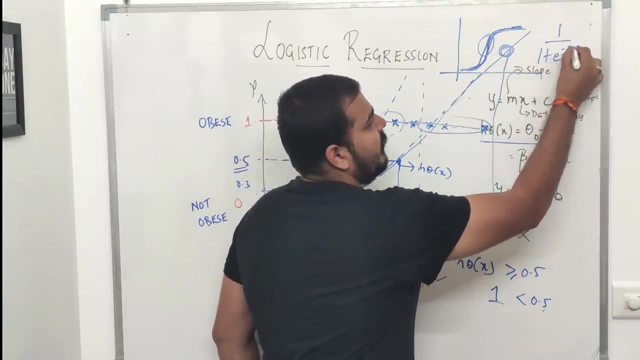 talk about logistic regression. it will create a line which looks like this, But we need to understand how this curve will get created. This curve is pretty much important. What is the math behind this particular curve? We can basically say that this straight line will get created with the equation 1 divided by 1 plus e to the power of minus x, which 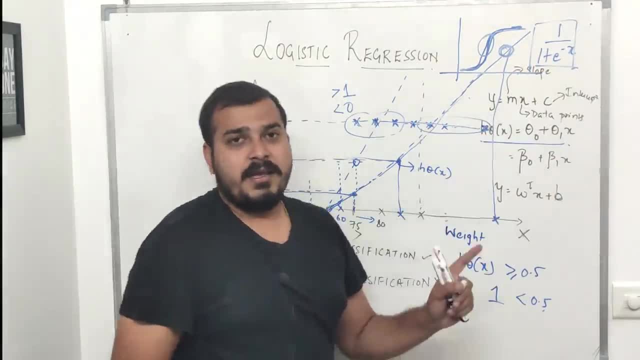 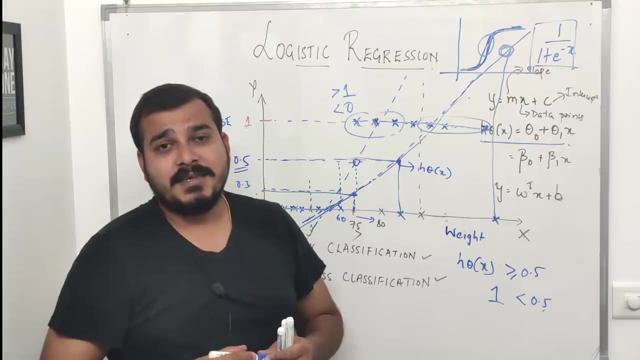 is also called as a sigmoid function. This is also used in deep learning, But how this particular curve is actually created, That we need to understand And that we will try to understand in the next class. So, before ending this particular video, guys, if you are looking for carrier transition advice towards 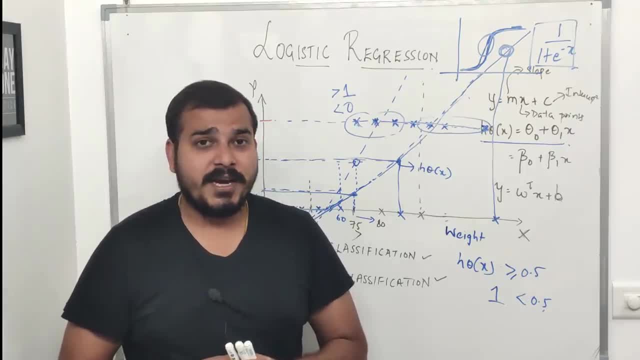 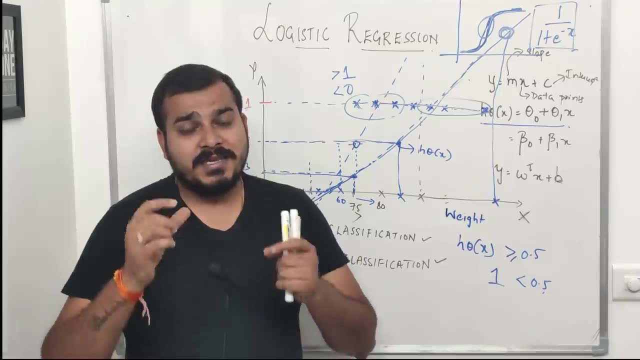 data science. please make sure that you watch the YouTube channel of Springboard India, because there you will be able to see talks of real world data scientists who are working in different different MNCs. The link is basically given in the description of this particular video.